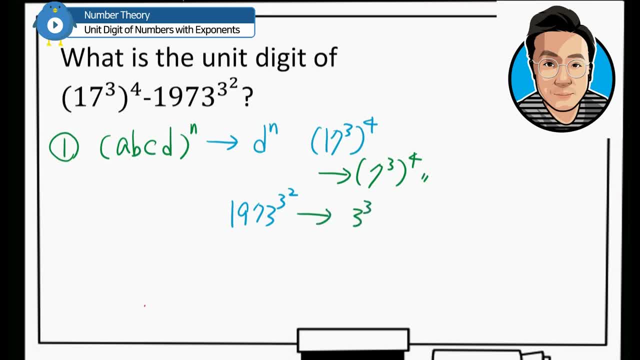 equal to the unit digit of 3.. to the power of 3, to the power of 2.. This is one thing we need to figure out. Then the second thing is for this operation of your exponent. So, if you take a look at these two terms, the first term, we have the parenthesis, We have the 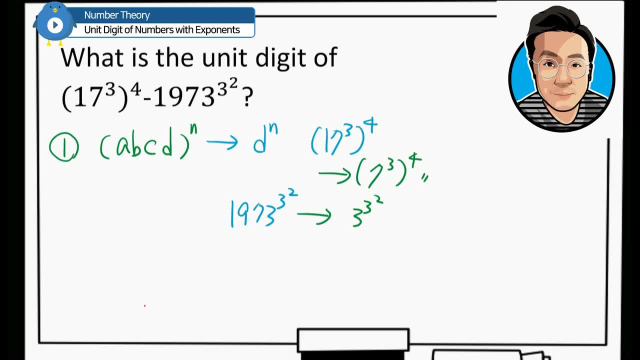 parenthesis, for the first term that means your base is going to be 17 to the power of 3 and your exponent of this whole thing has to be equal to 4.. So pretty much we need to use the multiplication rule for the exponent so that we can have 17 to the power of 12, but we do not have any parentheses on. 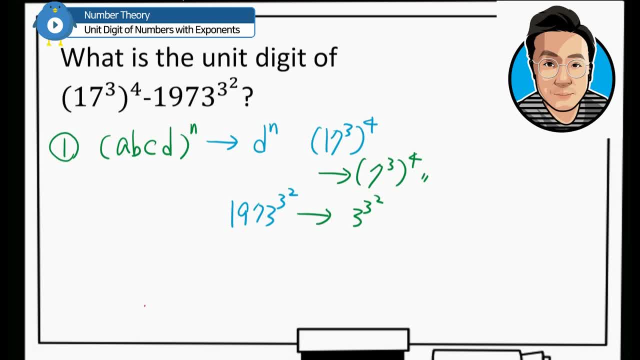 the second term, which means this 2, right here. this is only going to be the exponent of this number 3, which has to be another exponent of this 1973, so the second. we actually need to consider that, for example, a to the power of m, If you. 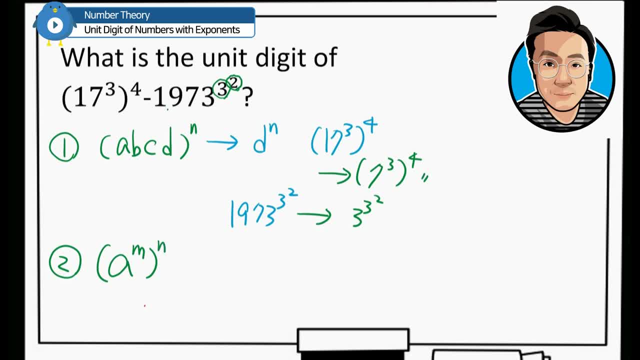 have parentheses with this. to the power of the another exponent, n. This is only going to be equal to a to the power of m times n. right? Then, at the same time, if we have this form without your parentheses, say a to the power of the m to the power of. 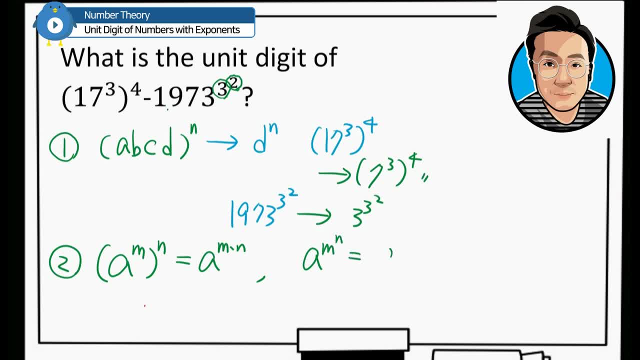 the n. This is only going to be, then, equal to a to the power of parentheses, m to the power of the n. Okay, this is what we need to consider, which makes our the first term. For example, the first term, the unit digit of 17 to the power of 3. 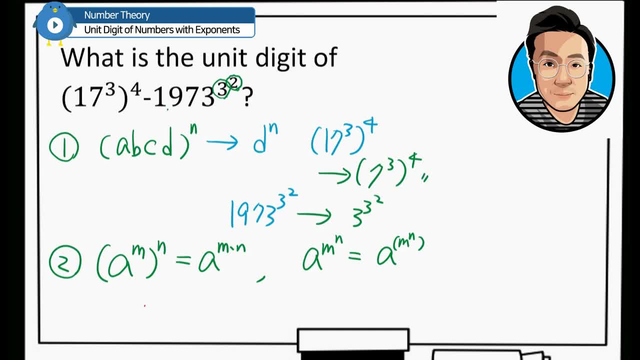 to the power of 4 is going to be equal to the unit digit of 7 cubed to the power of 4, right, So this 7 to the power of 3, parentheses 4, is going to be equal to 7 to the power of 12.. Then, what about the second term? So this 1973 to the 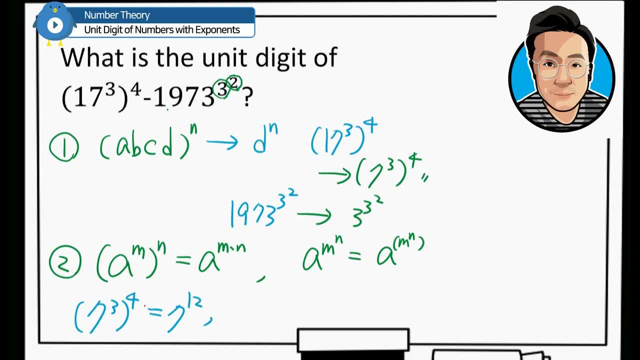 power of 12 is going to be equal to 7 to the power of 12.. So this 1973 to the power of 3 to the power of 2.. The unit digit digit of this number has to be then equal to 3 to the power of 3 to the power of 2.. So that's why this number 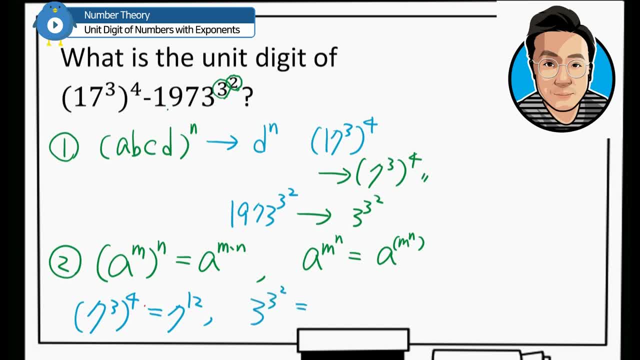 right here. This is then just going to be equal to 3 to the power of parentheses, 3 squared, which has to be equal to 3 to the power of 9.. We will be using these two numbers in order to find out about your unit digit. Okay, so, first of all, we need: 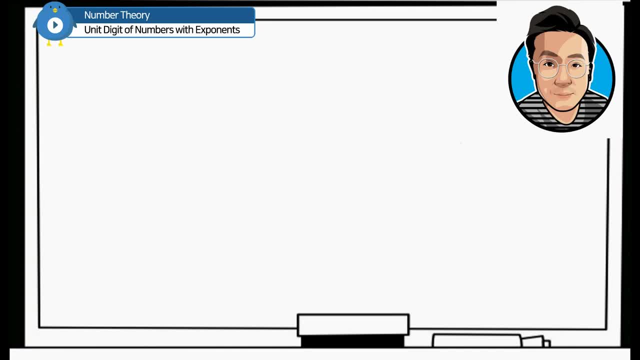 you have to find out about the unit digit of 7 multiples, For example. so case number 1.. Okay, 7 times 7 to the power of 1.. Just equal to 7, right, And what about 7 to the? 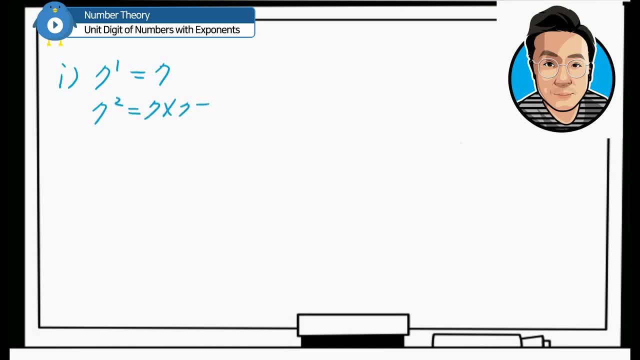 power of 2, which is equal to 7 times 7.. This is equal to 49.. What about 7 to the power of 3?? That is 7 times 7 times 7.. So the unit digit has to be equal to 7 to the. 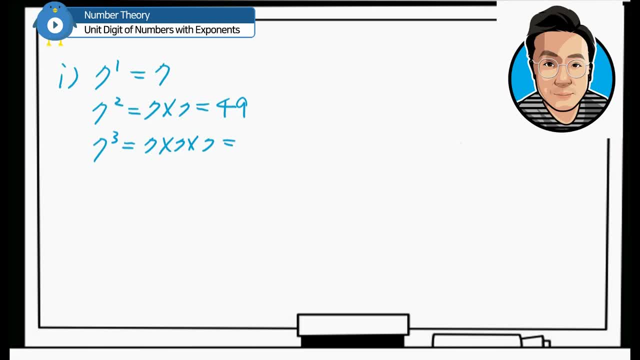 be then equal to 3, right, So the unit digit has to be equal to 3.. What about 7? to the power of 4,, which is then 7 times 7 times 7 times 7.. This has to be then. 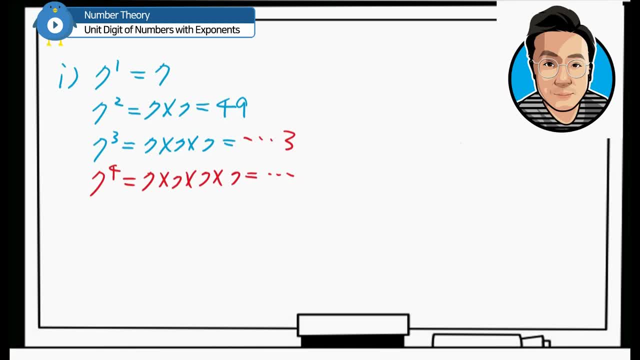 equal to some number with the unit digit of 1, right. So if you multiply another 7, which is 7, to the power of 5,, then the unit digit has to be going back to the 7 again, which means we have a pattern of 4, right, Okay. so the positive integer. 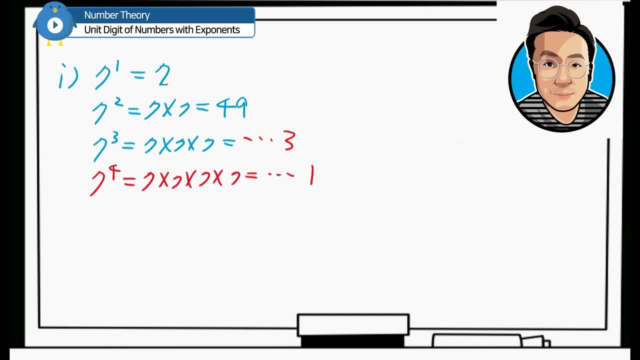 power repeats in pattern of 4,, as you can see right here- 7,, 4,, 3,, 1, then it gets back to 7,, 9,, 3, 1, and so on. Okay, this is case 4, 7.. What about the second? 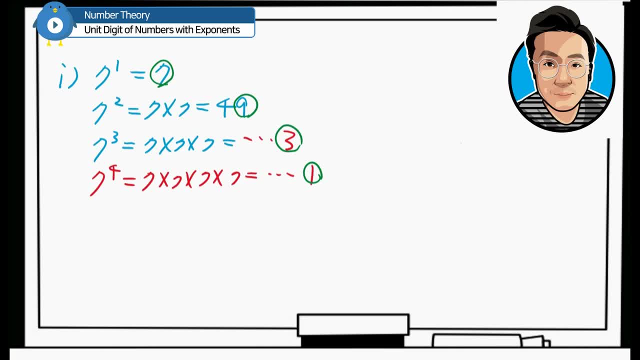 case. What about the case 4, 3? then? So case number 2.. Okay, this is case 4, 7.. What about the second case? What about the case 4, 3? then? So case number 2.. 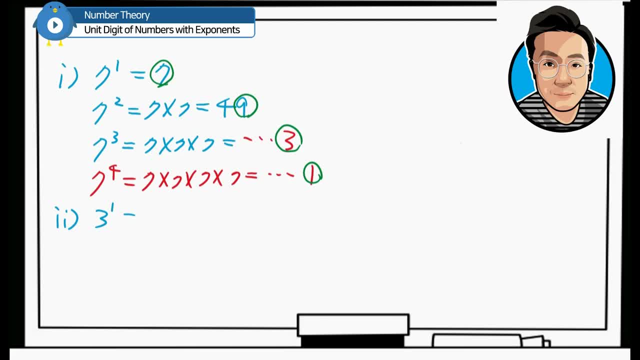 3 to the power of 1 is equal to 3.. Then 3 to the power of 2 is equal to 3 times 3,, which is equal to 9.. And 3 to the power of 3, which is 3 times 3 times 3.. This has. 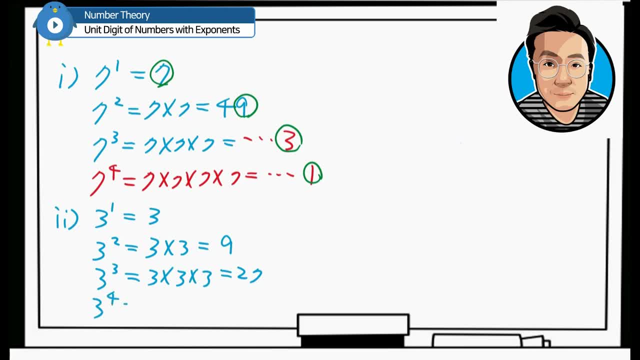 to be then equal to 27.. And 3 to the power of 4,, which is 3 times 3 times 3 times 3.. That has to be equal to 81.. Okay, so if you focus on the unit digit, we have 3,, then we have 9,, then we have 7,, then. 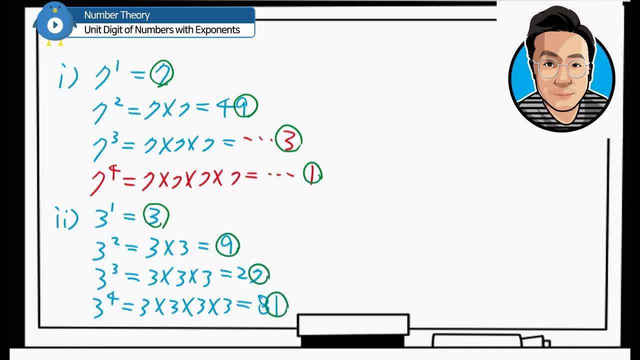 we have 1.. So another pattern of 4, so another pattern of the positive integer power repeats in the pattern of 4.. So we will be actually using this. So that means we can actually analyze this as what has to be the unit digit of the 7. 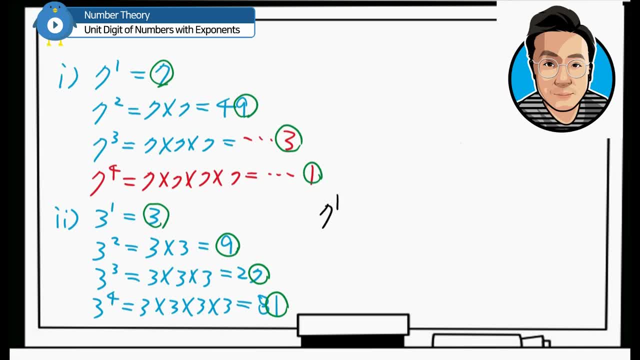 to the power of 12.. Well, 12 is direct multiple of 4,, right? So the unit digit of this number then has to be equal to 1.. What about 3? to the power of, at this time, 9?. 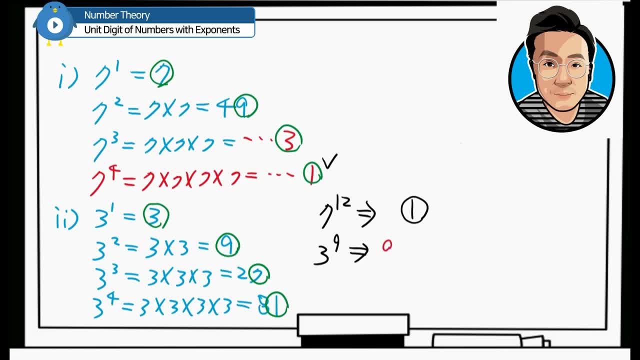 This case, right here, 9 is going to be equal to 4 times 2 plus 1, right, So after this, the pattern of 4, the positive integer pattern of 4, then we actually need to count one more. 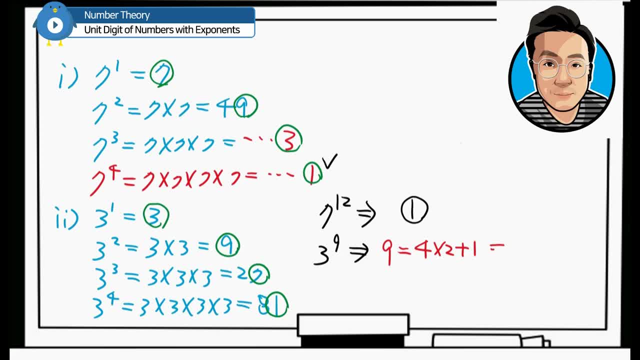 So that's why the unit digit of this 3 to the power of 9, has to be then equal to 3, right, Okay, so we're almost done, So we need to find out about the unit digit of this number right here, which is 17 to. 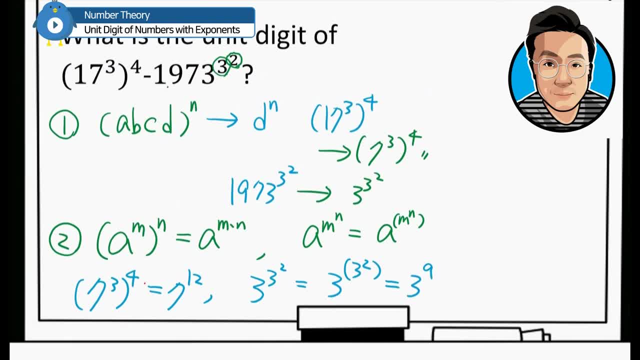 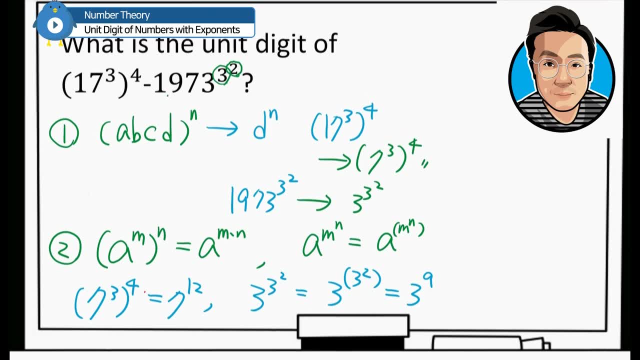 the power of 3 to the power of 4, minus 1,973 to the power of 3 to the power of 2.. So, basically, what we can notice is this number: the second term, 1,973 to the power of 3 to the power of 2, is much. 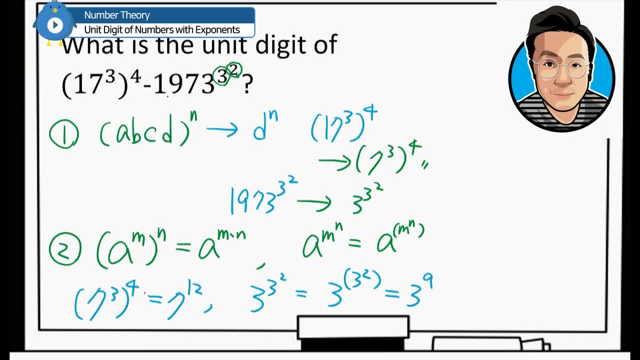 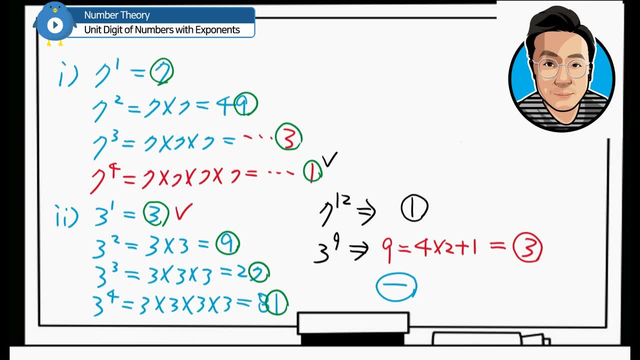 larger than the first term. So, whatever the answer this is, it has to be negative number, right? So it needs to be negative number. That safely makes us to say that your unit digit of the value has to be just 3 minus 1, which has to be equal to 2.. 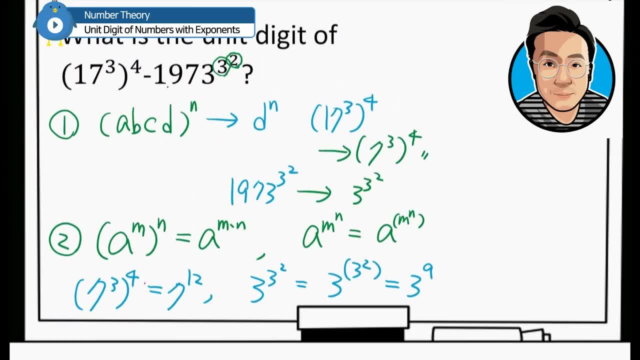 So the unit digit of this number right here that we are looking for has to be equal to 2, right? So that is the answer for this question.